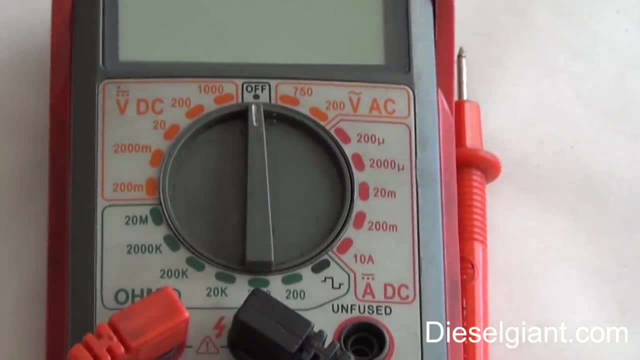 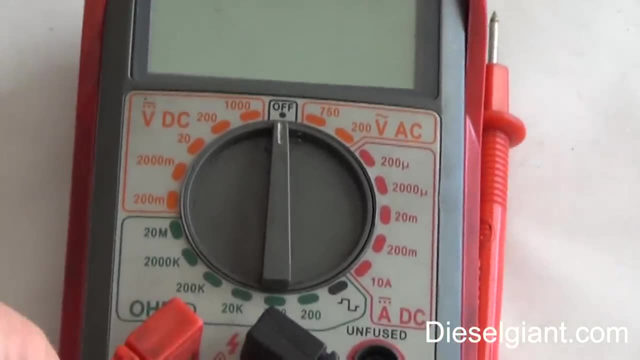 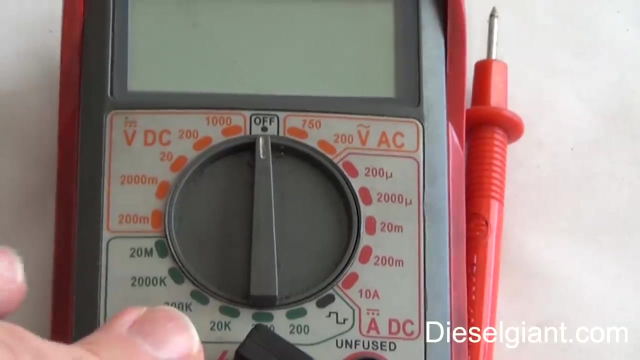 supply store like Advance Auto Parts, Pep Boys. You can buy them online. What I want you to do is I want you to get a good basic multimeter like this. It doesn't have to be fancy. These, I believe, are under about $30.. And this is basically all you need to troubleshoot. 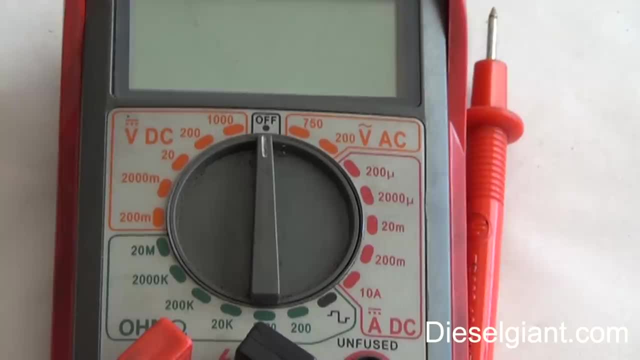 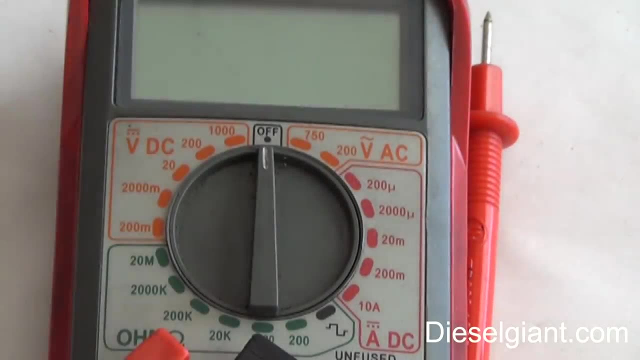 most electrical, common electrical problems that you're going to have on your car. I'm going to go over this just real basic And just try to give you a little explanation about what these different settings mean. Right here is what you're going to use on most of your automotive. That stands for volts. 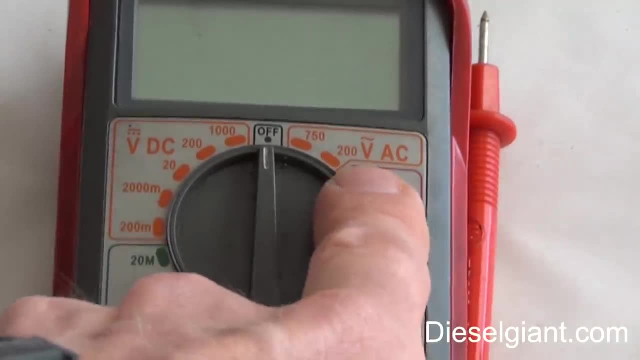 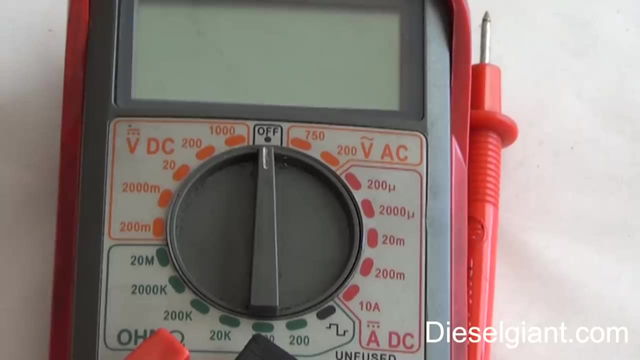 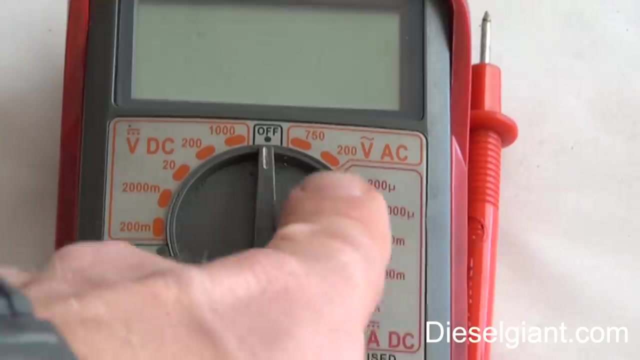 DC, which is direct current. Now AC is what you have in your house. In a nutshell, the difference in the current is direct current moves in one direction. The electricity usually flows from negative to positive. Now, on AC that you have in your house, it's called a. 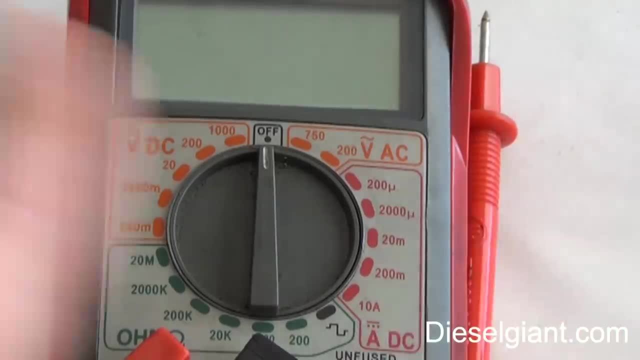 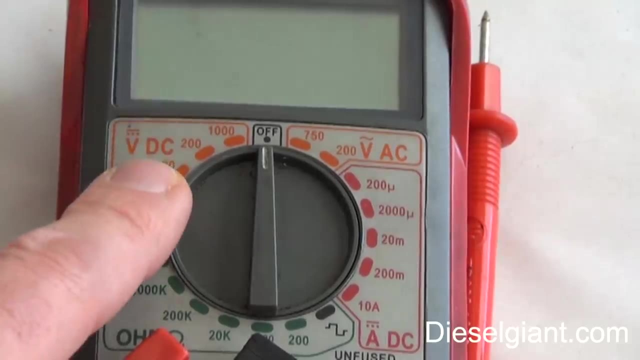 alternating current and it moves The electricity flows back and forth really really fast. That's all you need to know about that. Just know that the volts DC is what we're going to use on troubleshooting a lot of our electrical on our cars. Now you see, these got different. 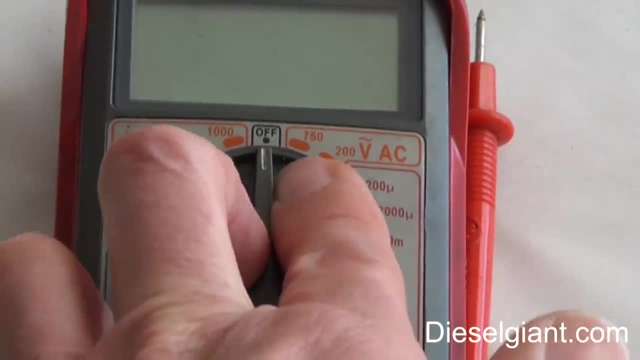 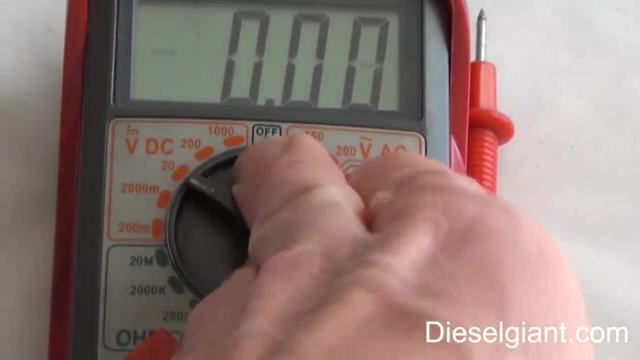 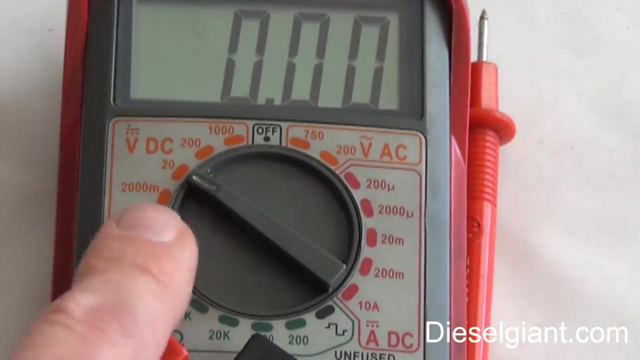 scales And usually when you turn it's basically moving the decibel for you If you get into the higher voltages. So what I usually use on a car is 20, because you're not going to get pretty much anything over 20 volts on anything. It's a 12 volt system, so this will. 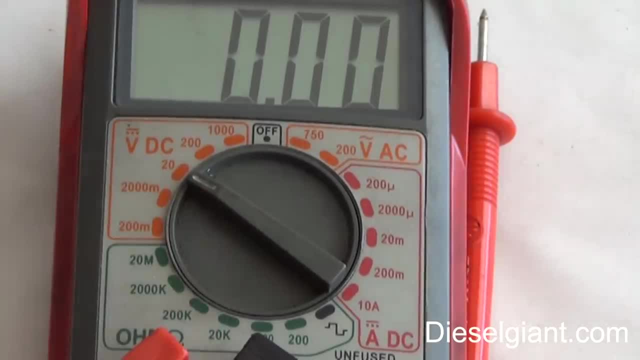 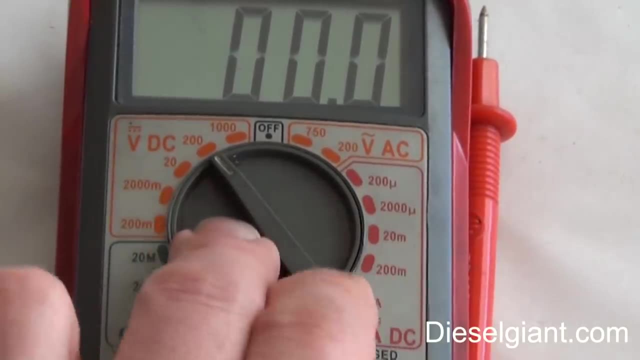 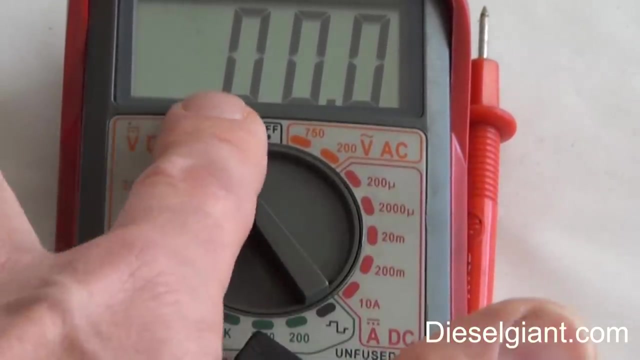 give you a good readout. So I usually use 20.. Your scale is probably going to. it may look a little different, but try to get close to 20.. We could use 200.. That would work also, But this way it'll give us like 12.25 volts instead of, let's say, 12.25 volts. So that's. 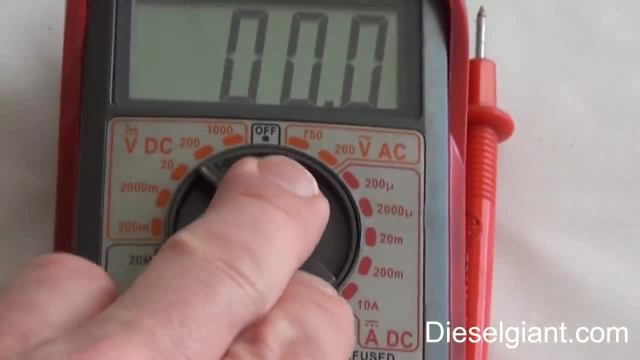 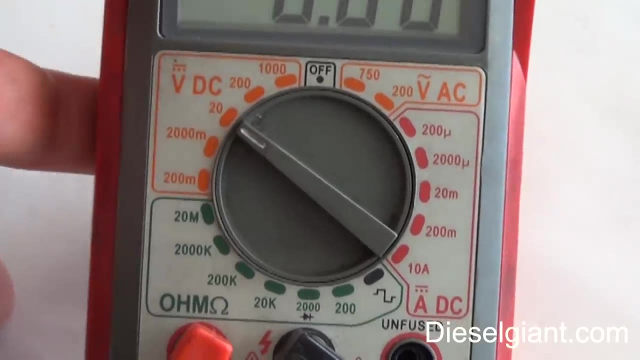 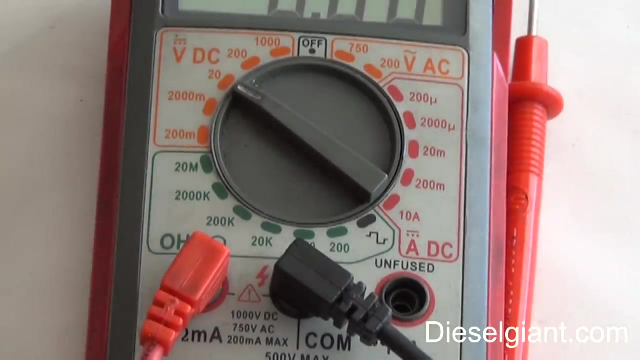 two or three volts, So it just gives us a little bit finer gradient to work with. Now, right here, you see, it says ohm and it's got that little symbol. It's like an upside down horseshoe. We're also going to use that for automotive work, to test resistance. Now, 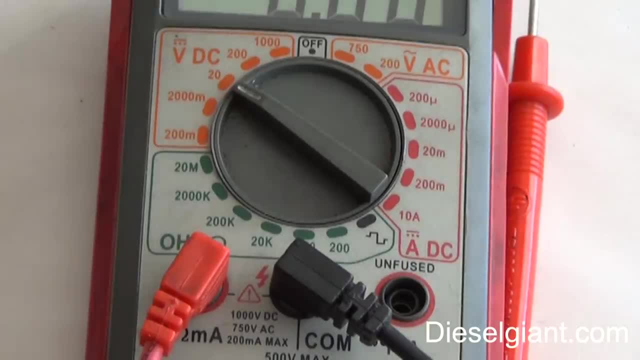 all resistance is? it means what kind of resistance to the flow of electricity? If you've got electrical going through, There's something that has no resistance, which there are always going to be some resistance. but the more narrow the gauge of wire, the harder it is to push electricity through it. 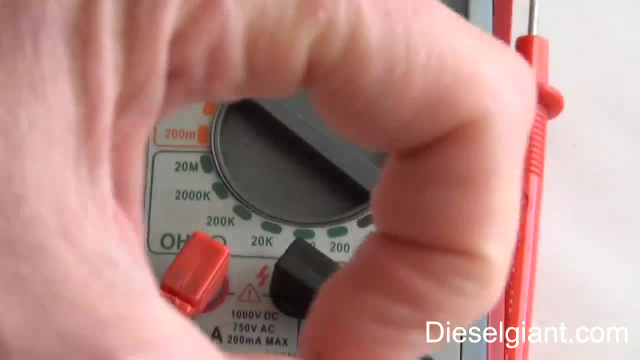 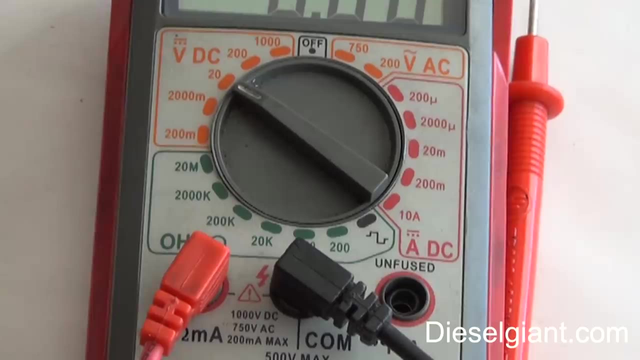 So that's how come you see battery cables that could be huge, okay, And you would think that those would have more resistance, but it's actually opposite: It's easier for the electricity throat to go through, such as your starting cables. a battery cable, that's. 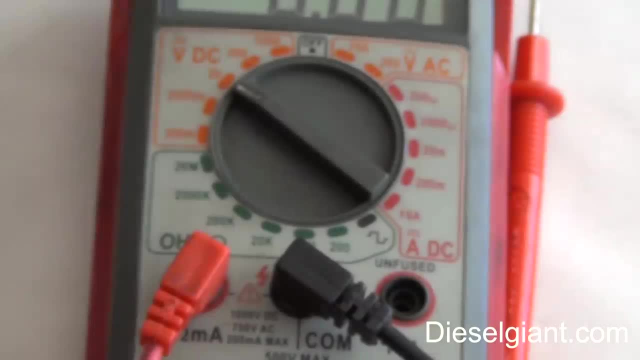 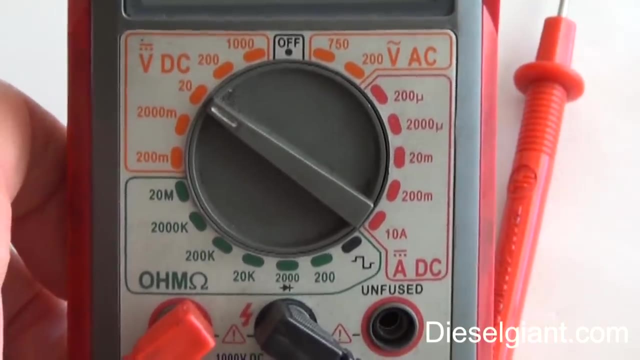 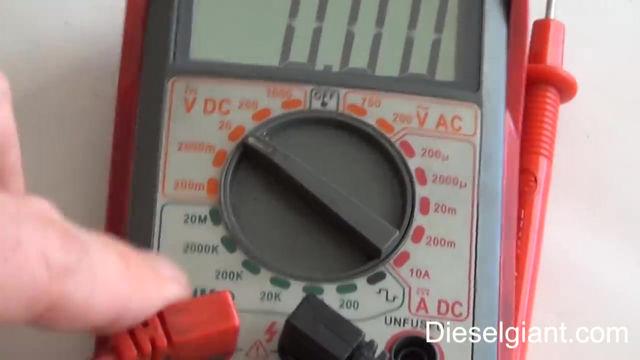 really big, as opposed to one that's really small, And I'm going to show you what these mean as far as with your car, So we'll not worry ourselves so much with the scale. But, as I said before, volts, DC and ohms- this is what we're pretty much going to be concerned. 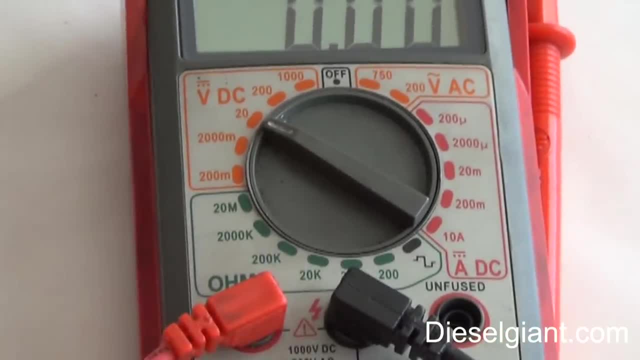 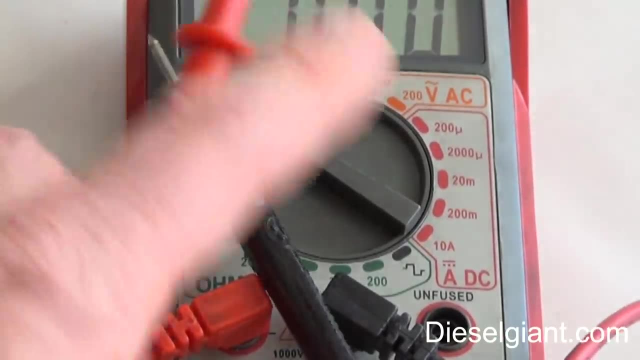 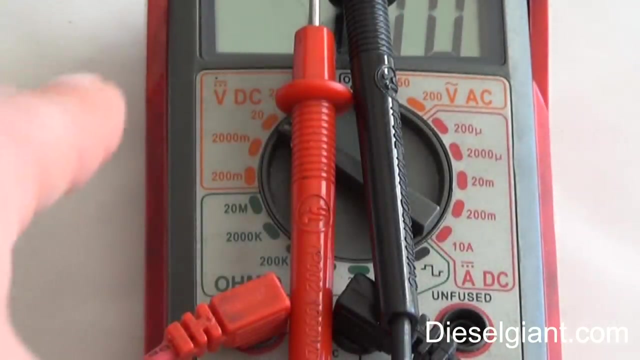 about today as far as doing some checks on your car. Now your leads- you're usually probably going to have a what's generally considered: this is the positive lead and this is the negative. Now don't be worried if you hook something up backwards, if you're testing voltage, because it'll just read with a minus sign: It's not. 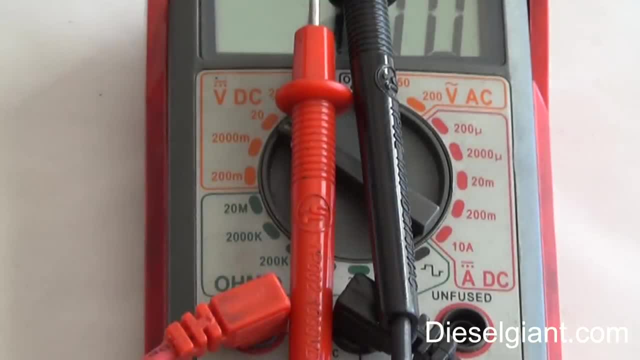 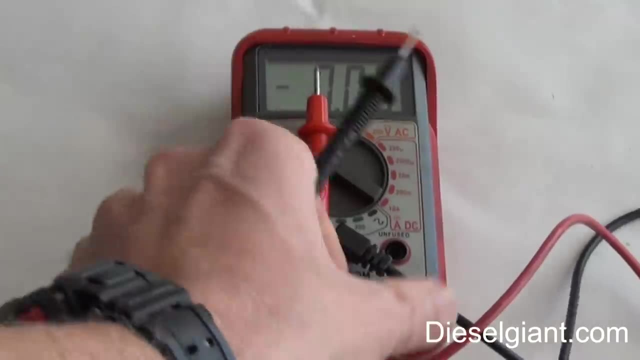 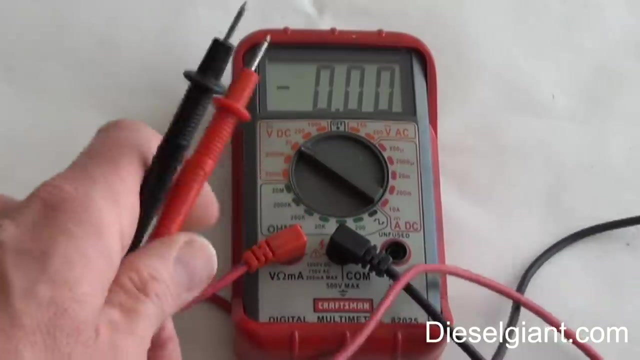 going to hurt your multimeter at all. What I do want you to be concerned with is I would like for you to make sure that any time you're testing voltage alright, you never put it on the ohms, because that could blow the fuse. When we're testing ohms, the meter has a battery. 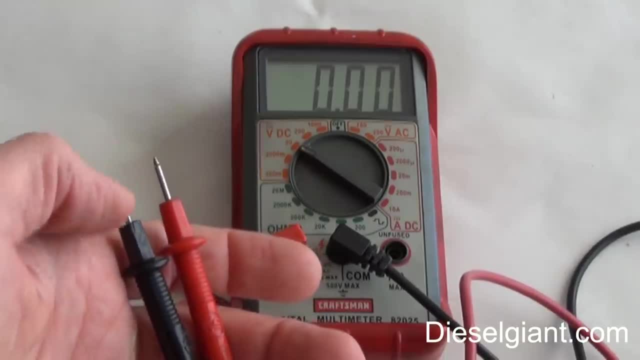 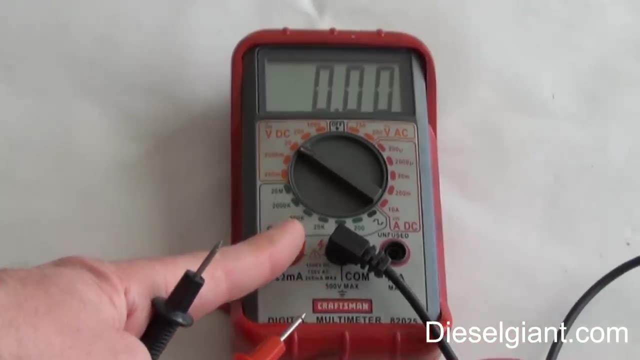 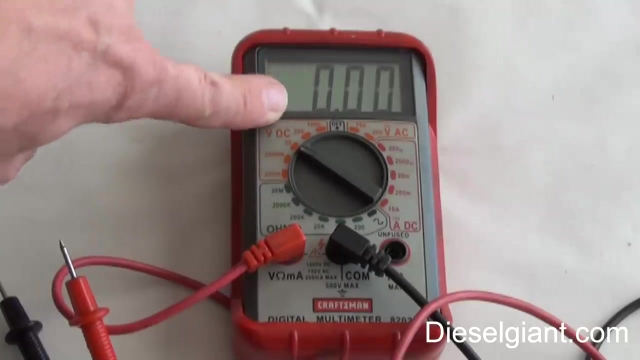 inside here that gives a little bit of electrical current so that we can test resistance. If we, let's say, have this to ohms and touch our battery, it could blow the fuse inside the multimeter and we don't want to do that. When we're testing volts, we're testing something. 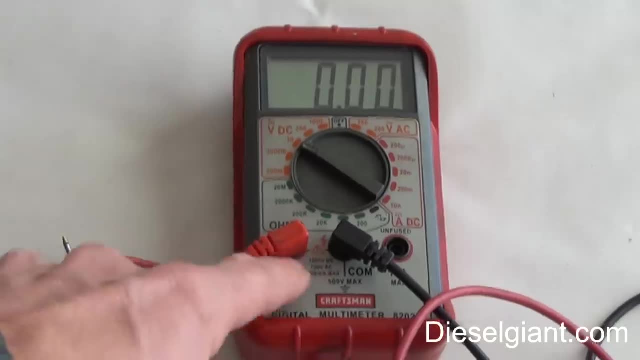 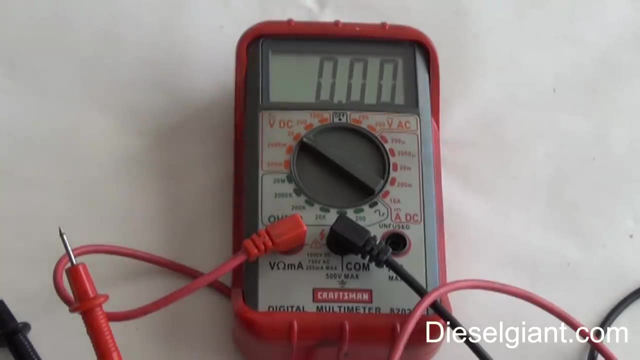 we're basically measuring electricity Here. we're measuring the resistance, This we're measuring the actual electrical power. There is a number of things that we're going to be concerned about. First of all, we're going to test what we've got in here. So let's go right over And over. here we're going. 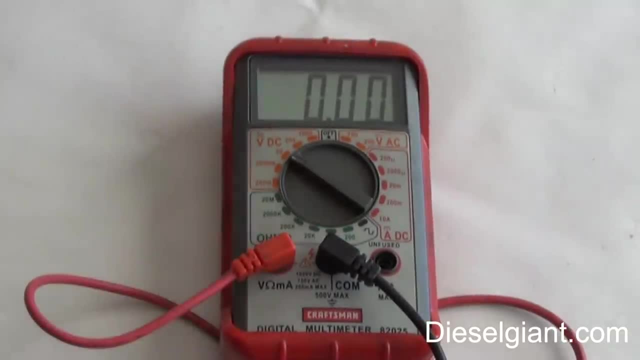 to test the AC. Another more important thing you can use this multimeter for is, as I said before, where it says volt AC, And that's what you would use to test, let's say, a plug in your house current. Please be very, very, very, very careful when you plug these in. 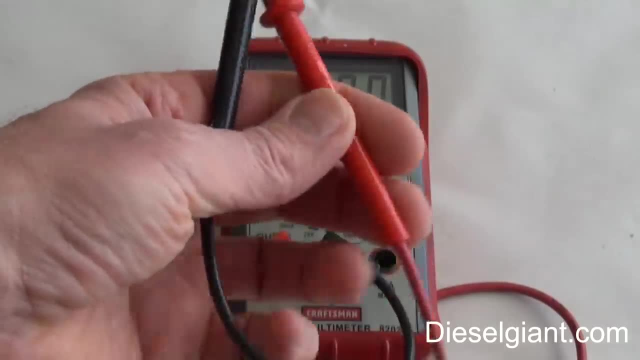 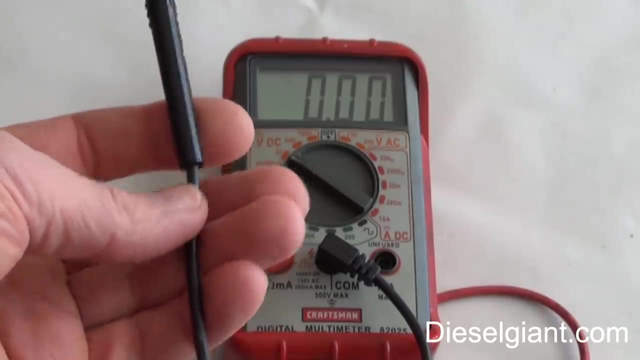 and I'm going to show you how to do that. But when you plug these in to a socket, make sure that you don't have any brakes in the wire. Make sure this is not cracked. This endém if one of these wires or something had a break in it and you were to touch your. 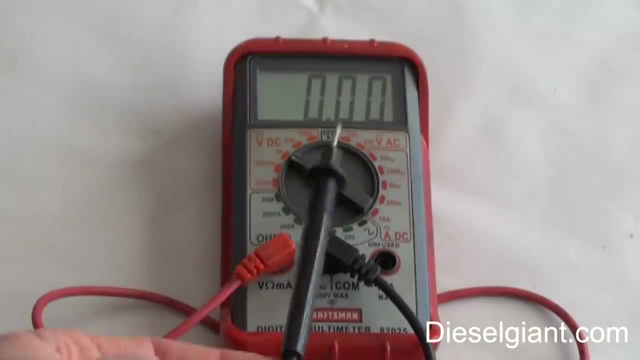 hand to it. under the right conditions, you could get a really nasty shock, and you don't want to get shocked from 120 volts- it hurts. so I'm going to set the camera up and I'm going to show you how to test the most common thing: automotive. 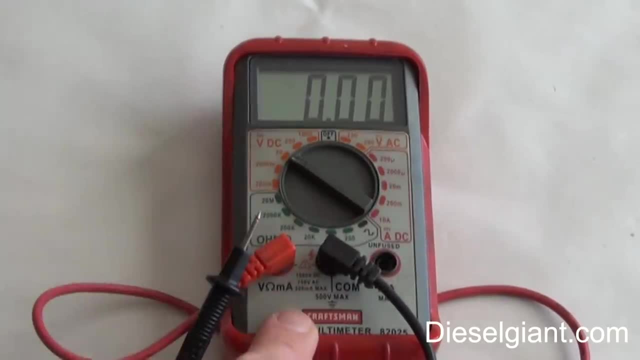 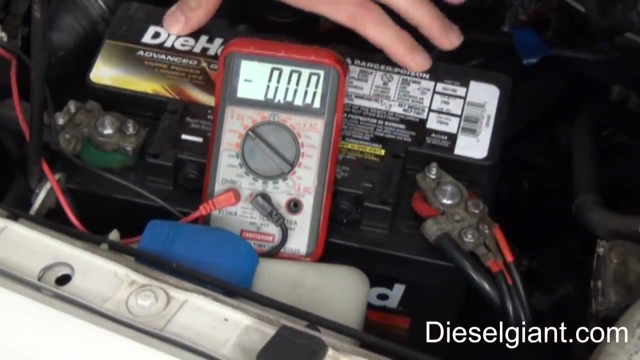 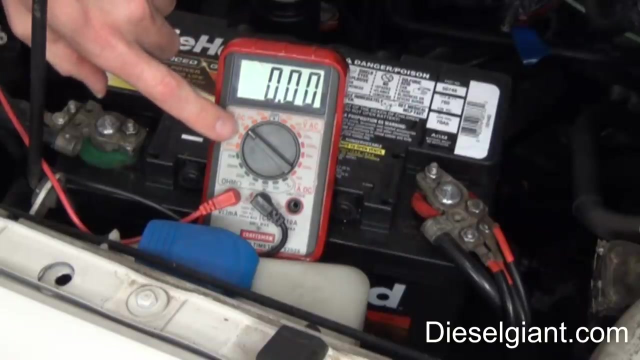 and the simplest thing- you probably first use your multimeter- is to test your car battery with. okay guys, we're going to test a car battery now. this is a normal 12 volt car battery that can be found in any type of passenger car. as I told you before, we're going to be checking volts and I have my gauge set. 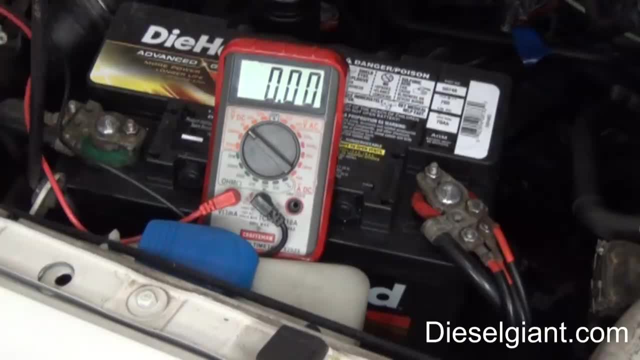 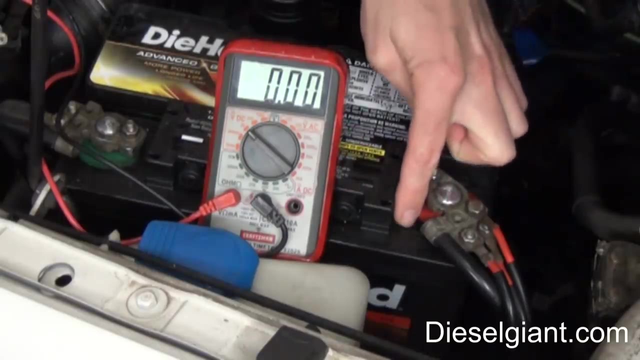 on to 20. so here's how we do this. you find which of your terminals is positive and which of them negative. normally you'll probably have a red battery cable or some type of indication, but please look on your battery. it'll have a plus symbol and where your negative terminal. 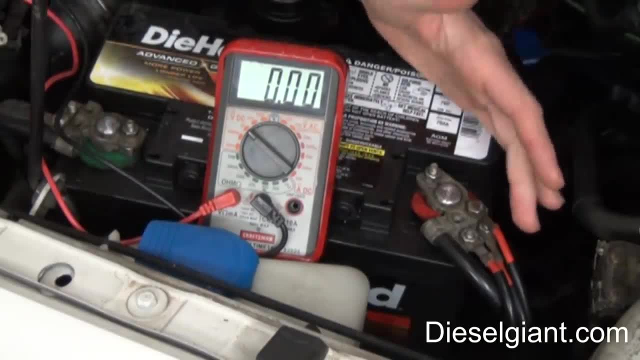 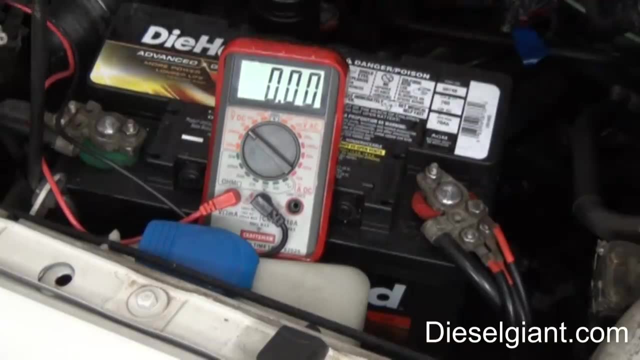 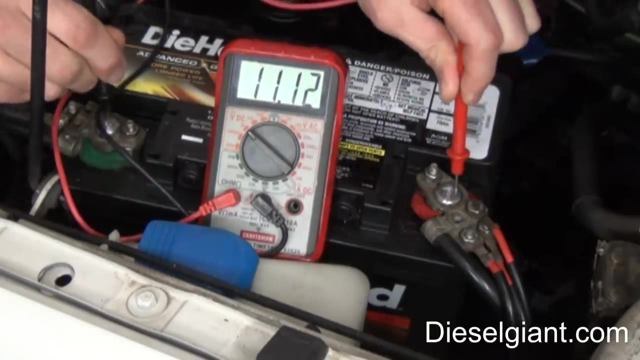 is, it'll have a minus symbol. so oftentimes the cables will be red on positive, but not always. and don't go by that. go by what it says on the battery. so we know that this sides are positive. we know that this side is our negative. so we're just going to touch the terminals, just like that, and read the. 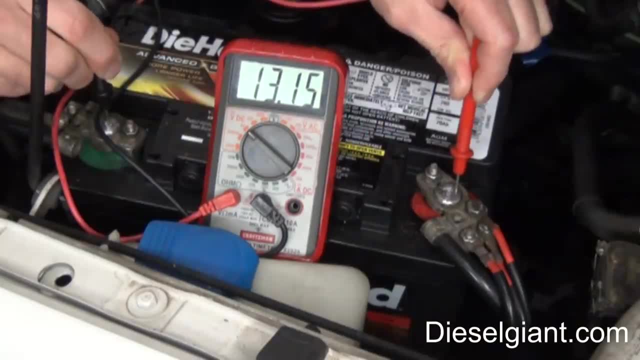 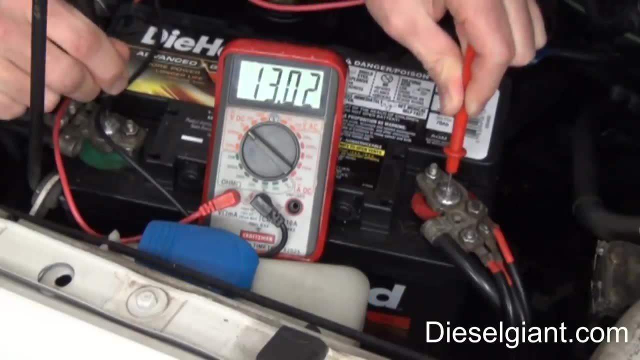 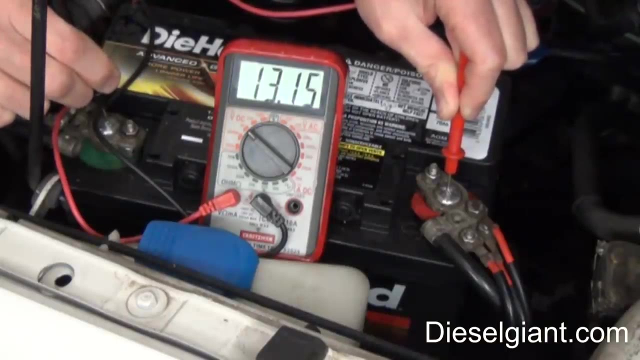 results. this says 13.15 volts. now you're probably asking yourself: why is this say 13 and not 12? well, if you're reading a battery and it says 12 volts, it's basically dead batteries. depending on the temperature, the air temperature, how cold it is, the battery will probably a fully charged. 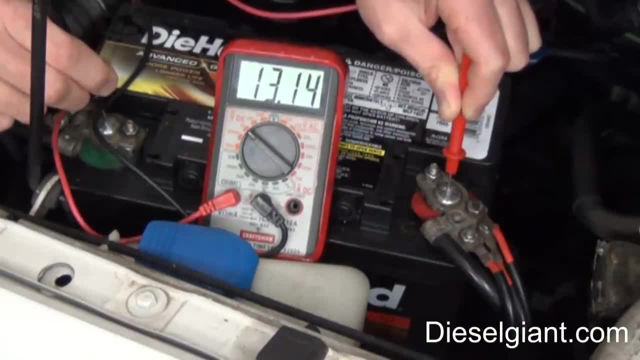 batteries about 12.6 to 12.7 volts. I've had this battery sitting on a battery charger because it's been sitting here in the shop for a while and I didn't want any type of degradation since it wasn't running, so it's just come off the. 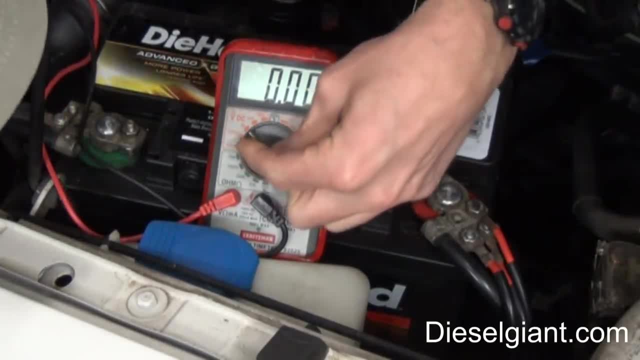 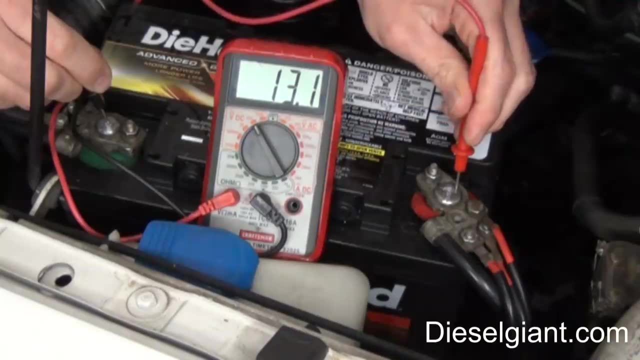 charger. so what I'm going to show you is: I'm going to show you the scale. we're going to switch it to the 200, okay, and see what happens when you touch that. it still says 13.1. all right, but, as I said before, try to get close to around 20 if 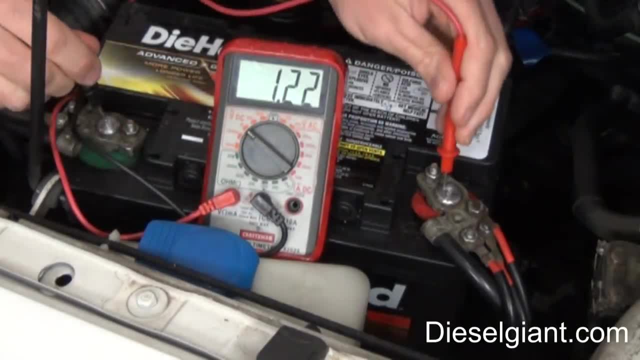 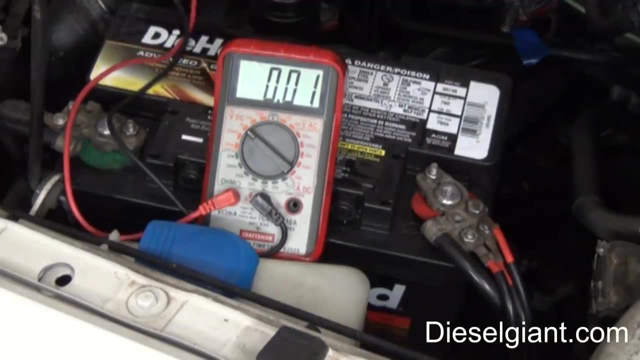 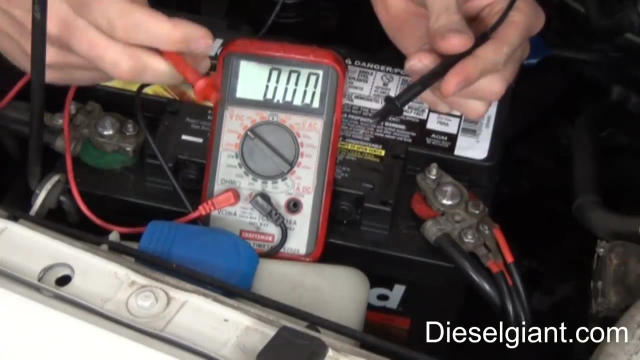 your multimeter has that, so it'll give you, give it to you in hundreds. so right there, 13.4. now, as I said before, what happens if you accidentally get the leads mixed up? all right, I've got the negative lead for the meter here. I've got the positive lead I'm going to touch. 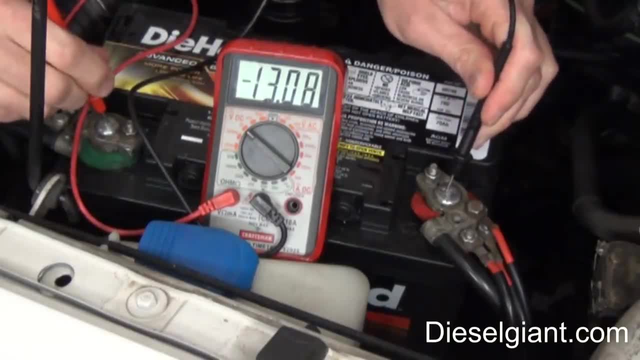 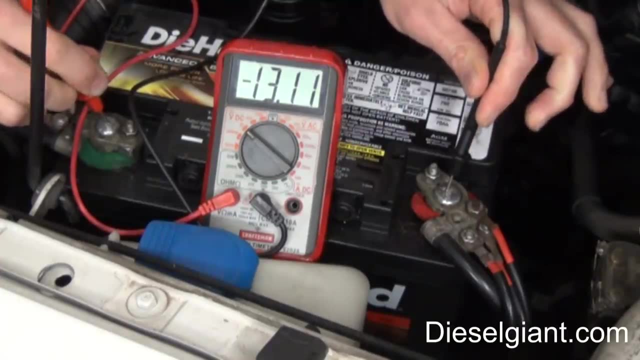 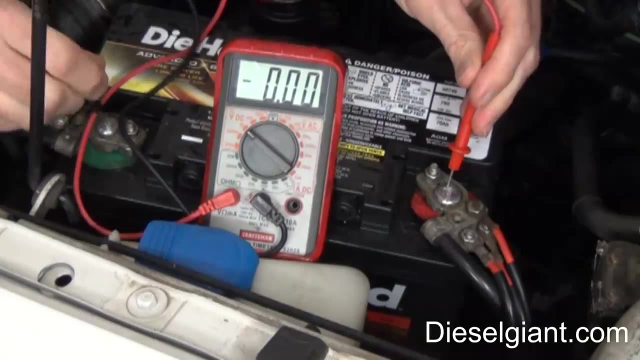 the negative to the positive, in the positive to the negative. you notice it still says yeah, about 13.10 volts. but you see the minus sign. it just means it's backwards. it's not going to hurt the meter at all, okay, and we just go back and do it like this. okay. now, what you don't want to do is you don't want. 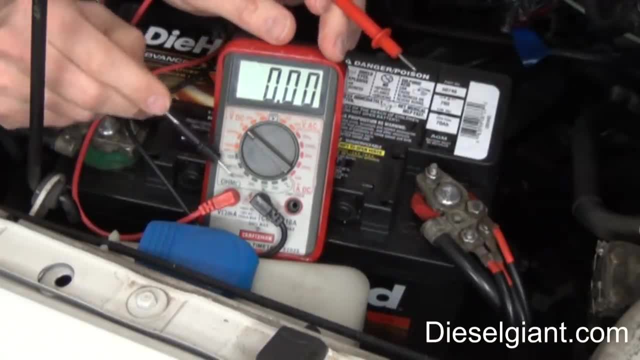 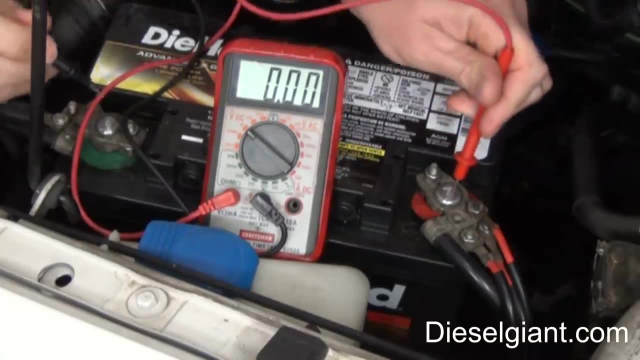 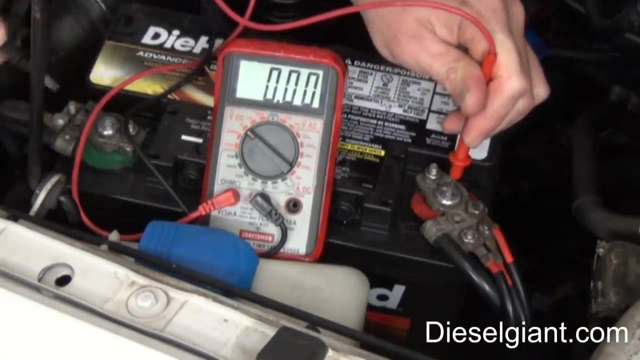 to touch the oh ohms when it's on ohms to this, it would probably blow the fuse in this multimeter. okay, so that's the first test. your battery test now. if you were to run your engine, it's going to read a lot higher. it may read about 14.5. that's because the alternator would be charging the battery as the 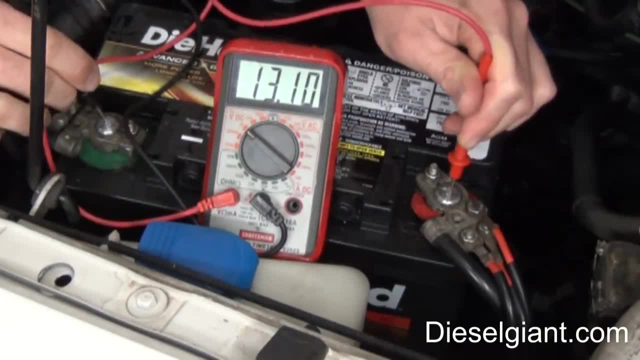 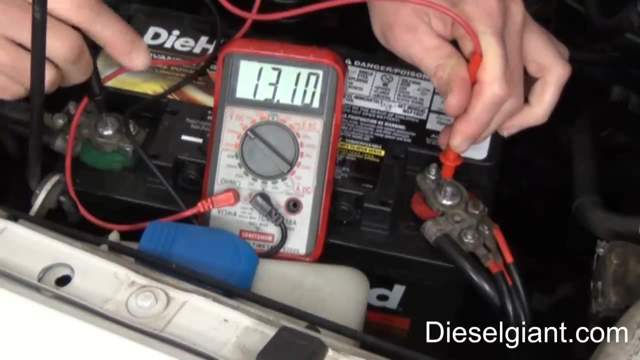 engine's running. so if you want to test your alternator, just have the engine running and touch same thing. touch the terminals to the battery terminals and you're going to see what kind of voltage your alternator is putting out. if your vehicle's running and you don't see any additional, 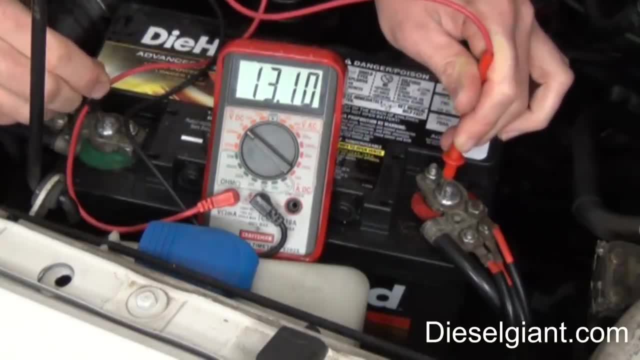 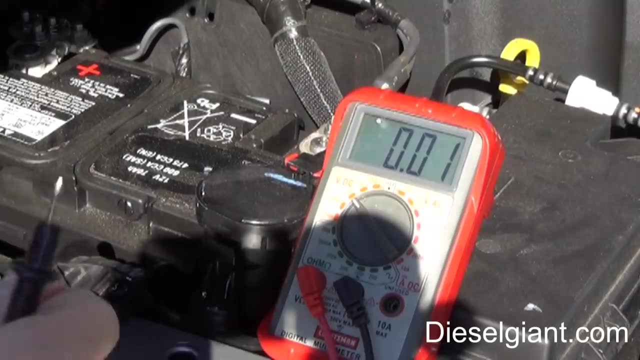 voltage, and that means your alternator is not charging, and you know what. i can tell you this, but actually i want to show you this on a different vehicle. all right, hopefully the wind is not going to be too bad while i'm out here, um so let's test this battery. that's outside. 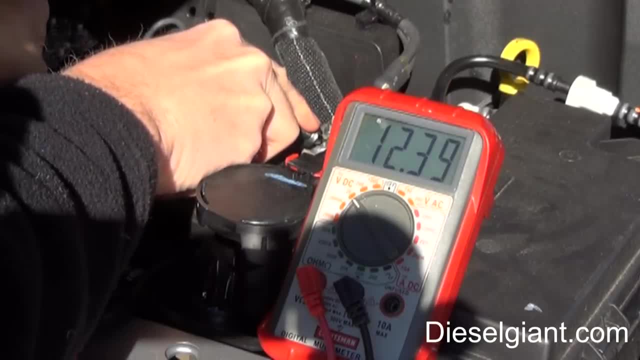 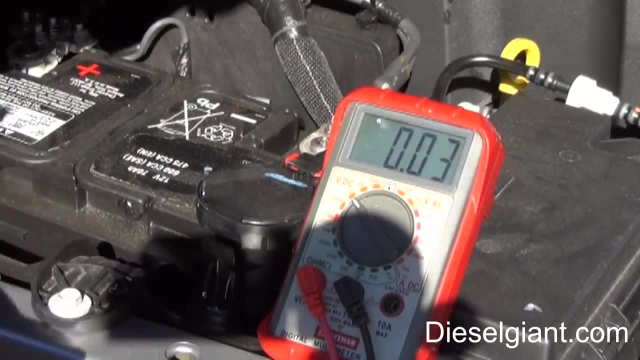 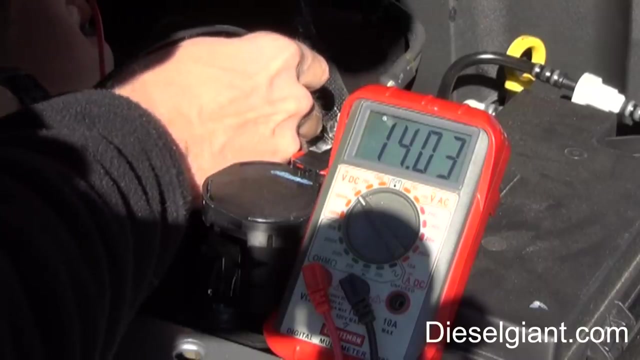 and we see we get 12 point 12.39 volts. now i'm going to go ahead and start the engine and we'll show the difference in the voltage when it's running. all right, with the vehicle running. you see, it now says 14 point about 14.2 volts. 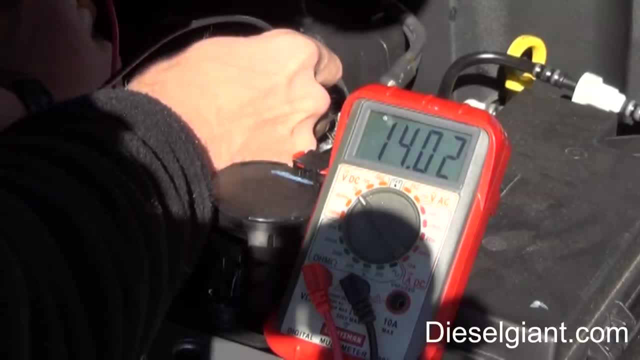 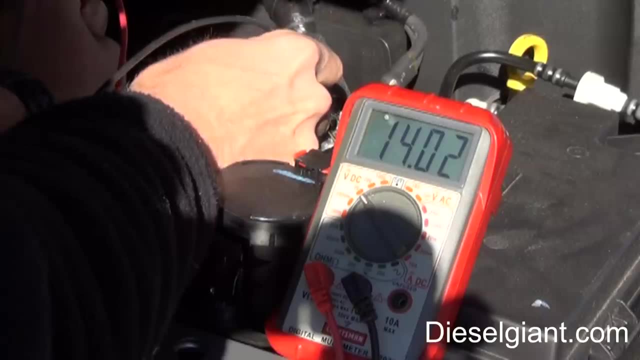 so we can see the difference in when the vehicle is off and it's on. so this is a good test if you're not sure if your alternator's charging or not, so let's test this out: charging um, if you're trying to track down a problem, it's something that anybody can do. 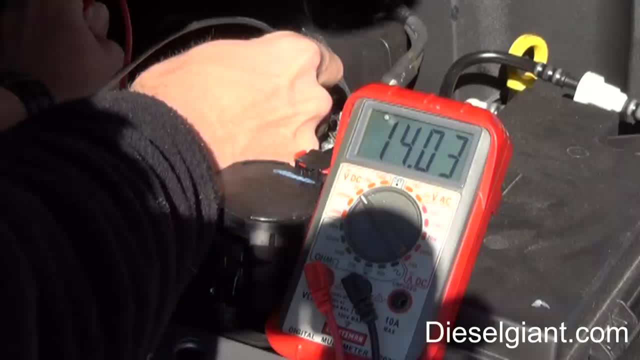 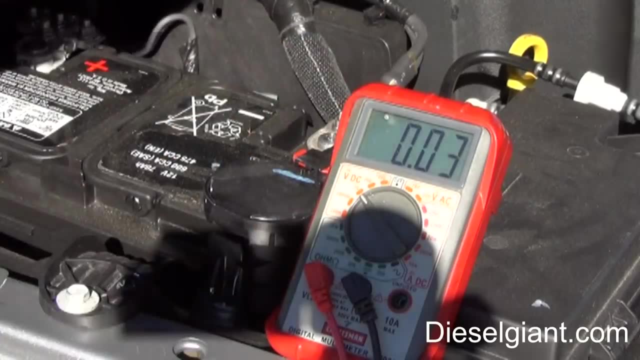 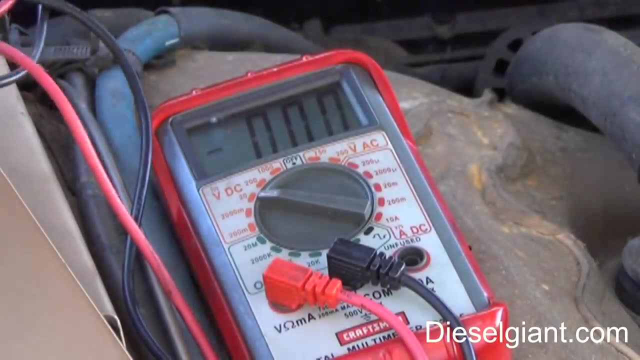 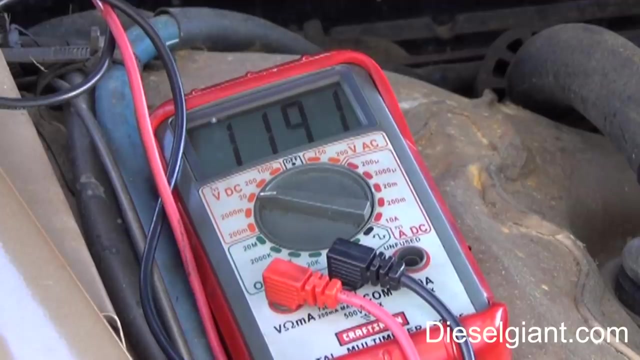 this alternator is putting out basically 14.4 volts right now, so it is in a proper working condition. i just realized that i had a battery here that will not start the car and i wanted to show you what the voltage is. all right, see, this battery is reading 11.3. 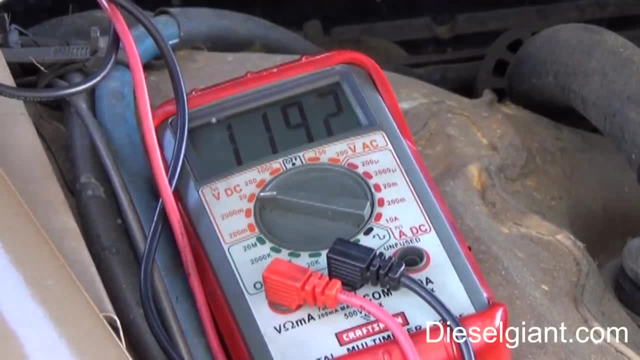 volts, you would think, because it's near 12 volts, that it's good, but this battery is completely um, at the end of its life. it will not start the car and it won't hold a charge. one other quick test that i wanted to show you about checking batteries. it's not just related to 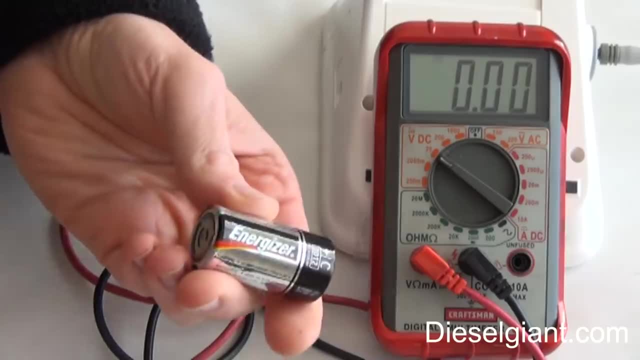 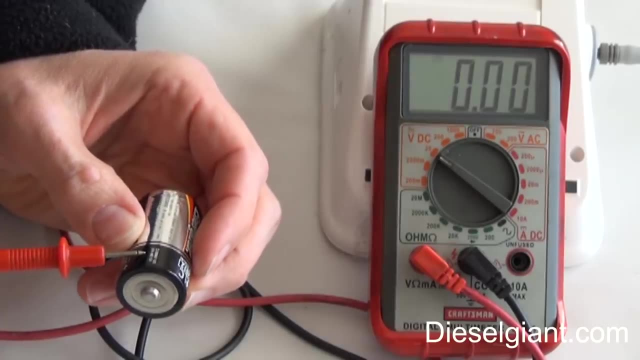 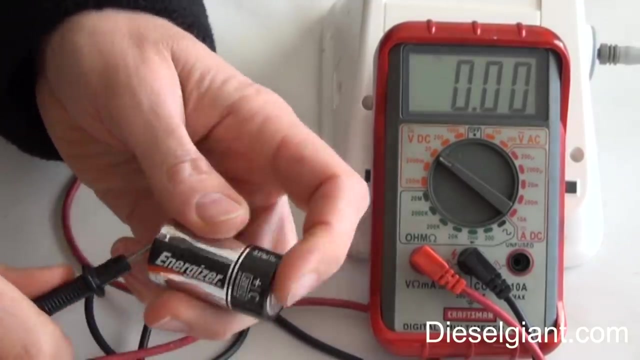 automotive. you can check any type of battery that you have around the house. this is a c cell and this is supposed to be 1.5 volts. just make sure to set that to volts. so of course it's got positive and negative, so we're just going to hold the leads. 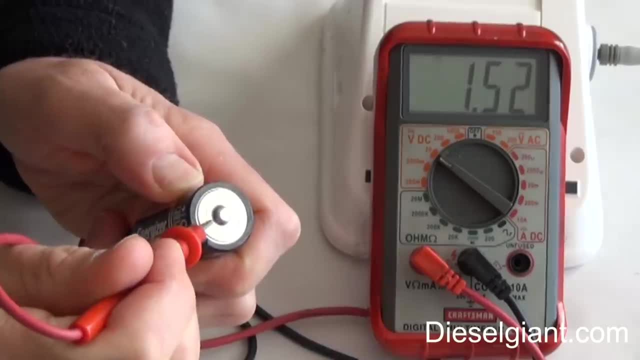 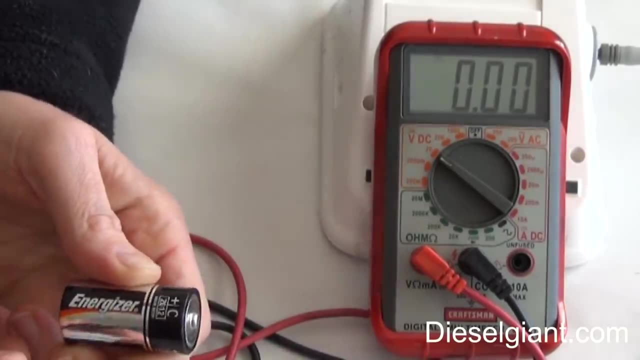 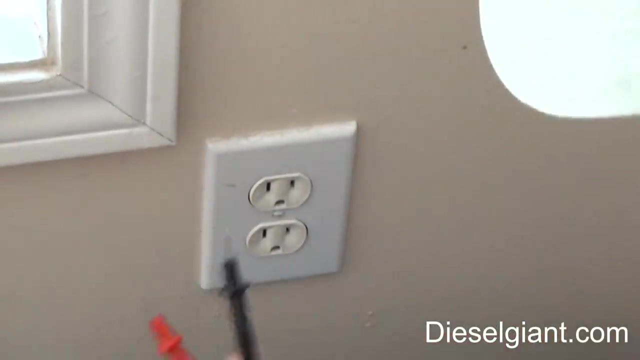 like so, and we're going to see what we read. all right, we're getting 1.52 volts. so if you've got 9 volt batteries, double A, triple A, doesn't matter, just make sure to set this to volts dc. okay, and speaking of house current, i promised i would show you real quick how to set this current up in a dollar little bit. 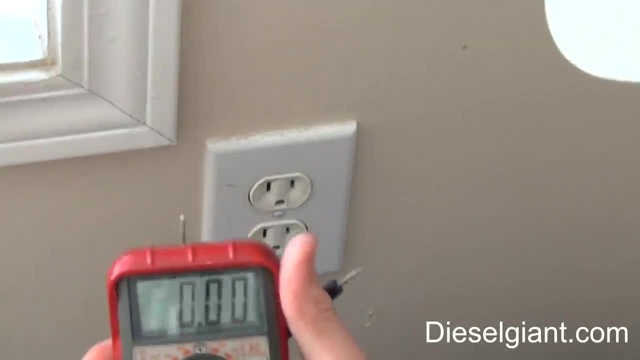 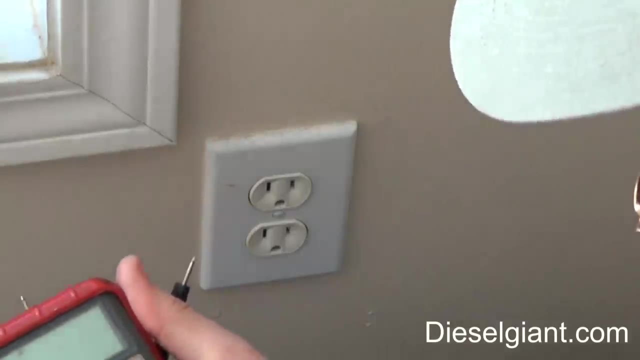 so the reason for this is that i'm seeing a lot of work here. i need to really get my good power into the alternator. you real quick how to test for current in your house. again, you're going to put this to volts AC and my scale has 200 or 750 and we know this is going to be 110. 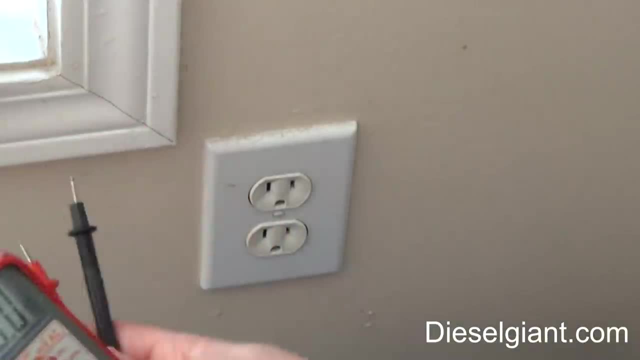 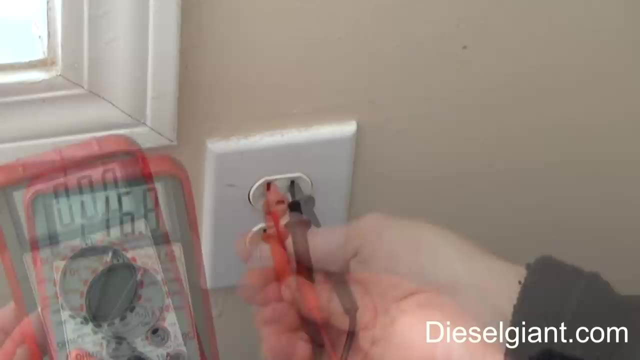 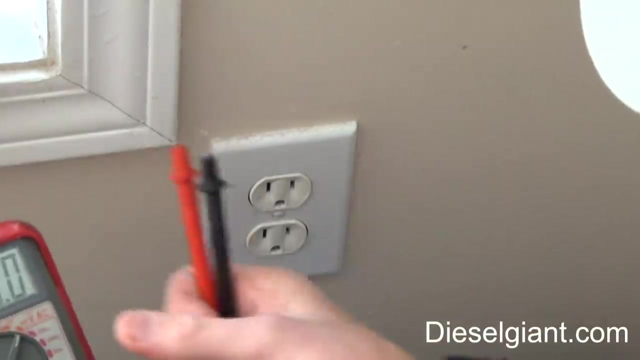 or 120. so I'm going to turn it to 200 and I'm going to take both of my probes and put them in. just ok, raise 118 point 4 volts, all right, so that's normal house current. again, since this channel is automotive related, don't go around. 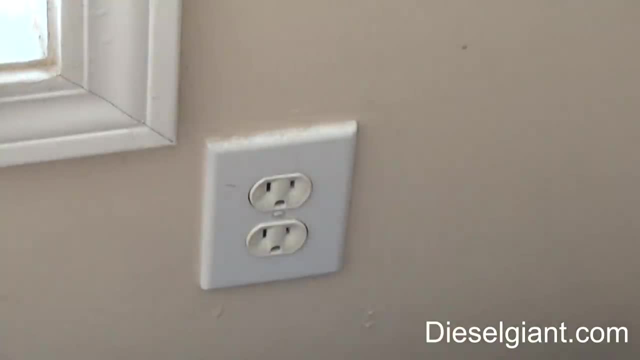 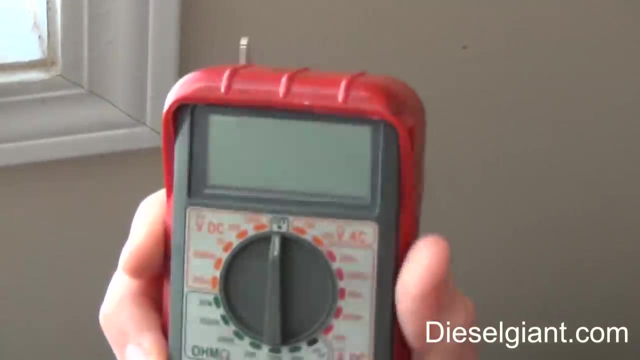 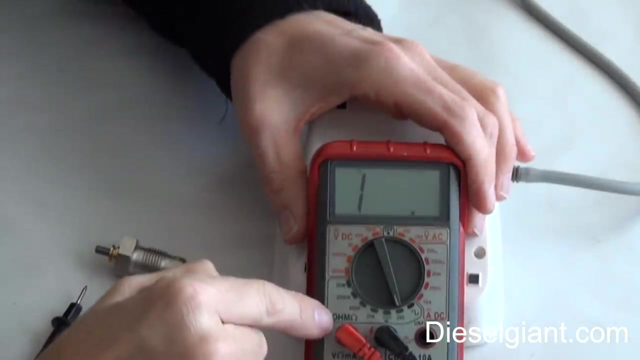 sticking these in you, in your current- okay, in your, in your house. it's just dangerous, all right, so now I want to show you how to check resistance. okay, now, I promised you we're going to check and show you, you, how to do resistance. now again, I've set my scale on the ohms to. 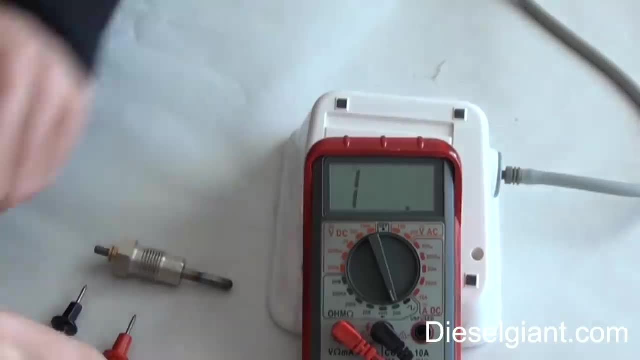 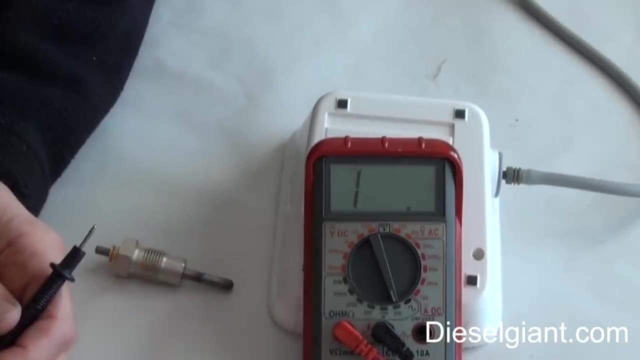 approximately 200. all right, so basically, if you see your display like this, it's just got a one or it may be it may have a little symbol on it. that means it would be the same thing as if there was a short okay, or you can say the circuit. 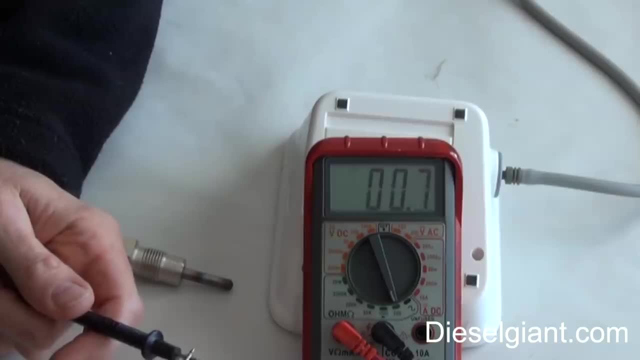 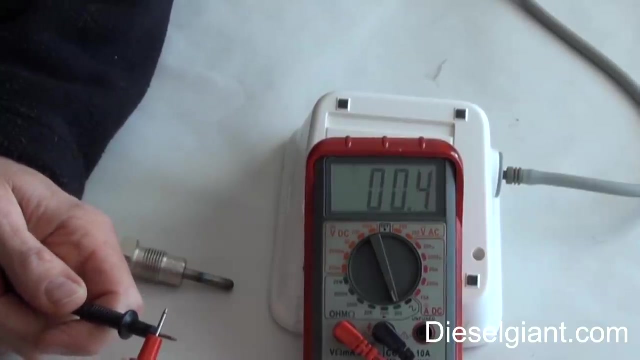 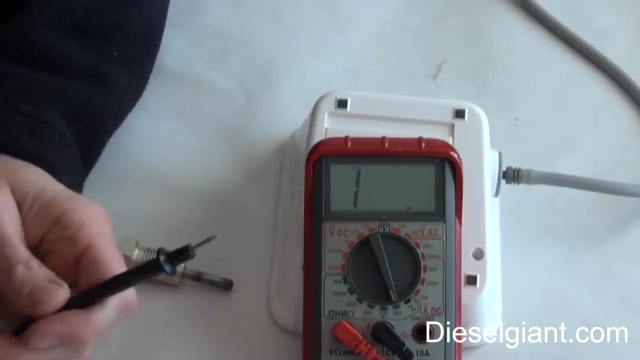 is open. now, if I touch the two wires together, what it's doing? this meter is sending a small amount of electrical energy through the meter and it's reading the resistance of the probes and the wire. all right, so you can see it says 0.4. that's 0.4 ohms of resistance. now there, anytime you have something. 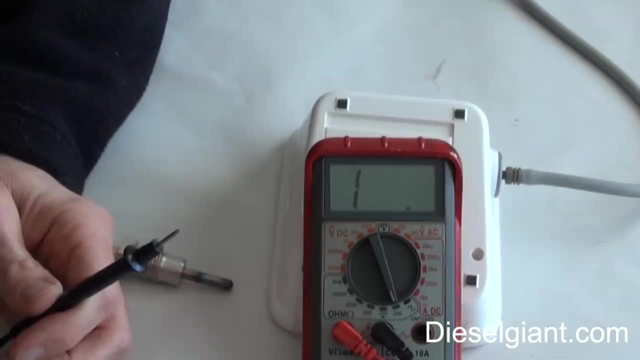 that electrical energy is going through, you're going to have some resistance. it could be so. my new your meter couldn't pick it up, but we do know this is standard for this for this meter. your meter may read something a little different, but 0.5 or 0.4 ohms of resistance between these two. 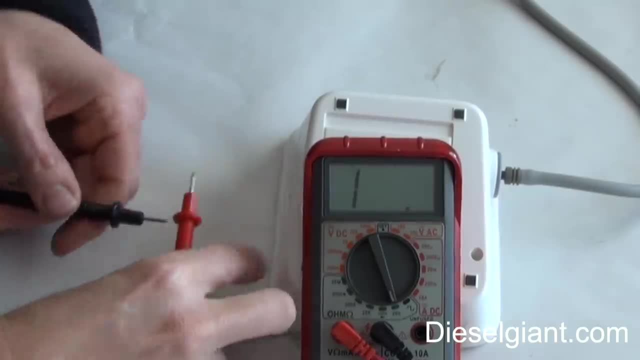 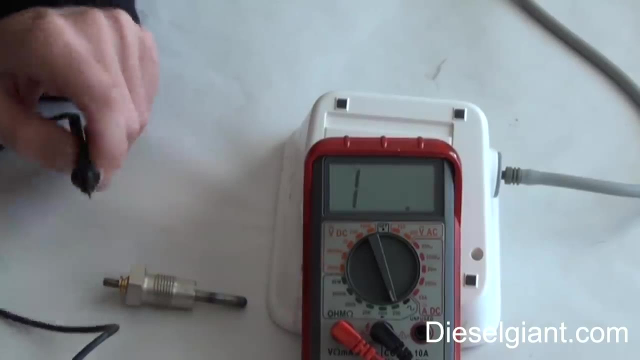 wires. now again, if you're testing something like, if I'm testing this plug and it reads this, then that means there's a short or there's an open, though it could be the wires broken. so if we wanted to test this glow plug, I'm gonna put one of my leads. 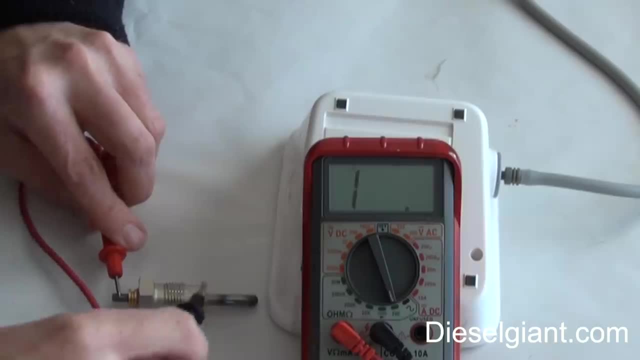 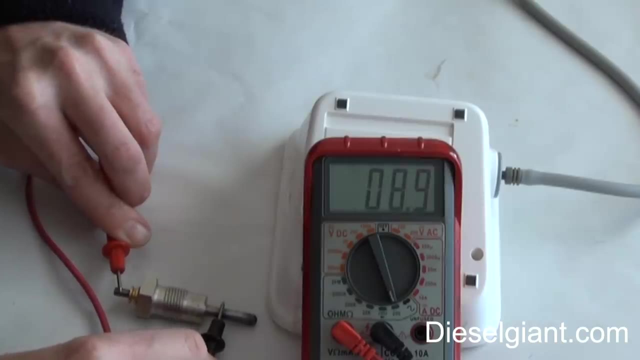 where the power would go in, right here, The power wire would connect here and then I'm going to check the other end of the plug itself. All right and we're getting. and the reason it's bouncing around is because I may not have a good connection or I may not have. 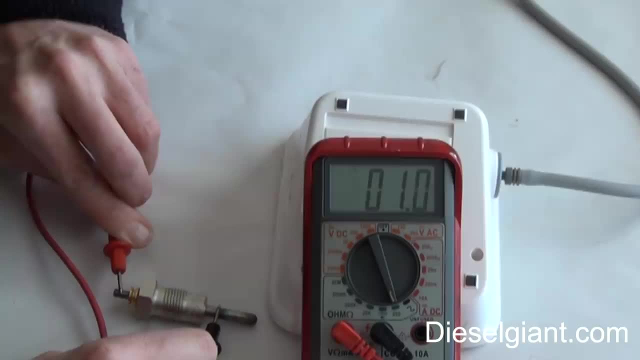 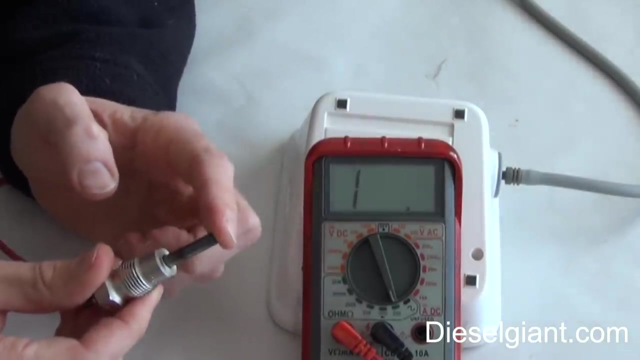 it on there real good, but it's reading about 1.5,, if I can hold it, still about 1.5 ohms of resistance. Now, remember the reason that this can glow. this is a glow plug. the reason: 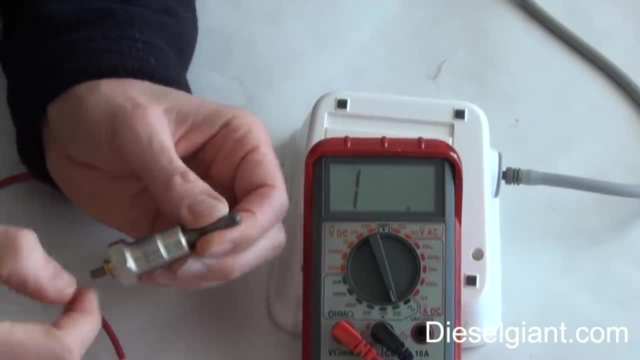 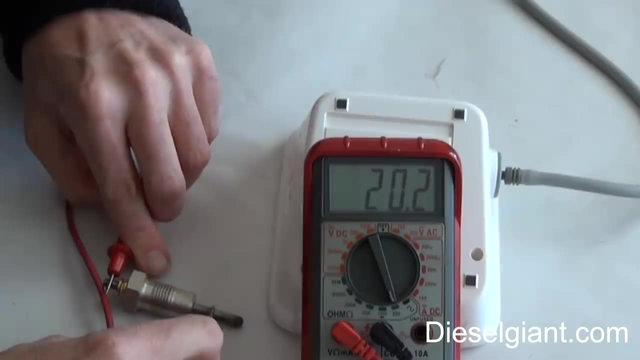 that this can glow and get hot is because there is resistance between here and here. okay, So if I asked you to test your glow plugs, when you test your glow plugs, you're going to get a lot of resistance. So if I asked, 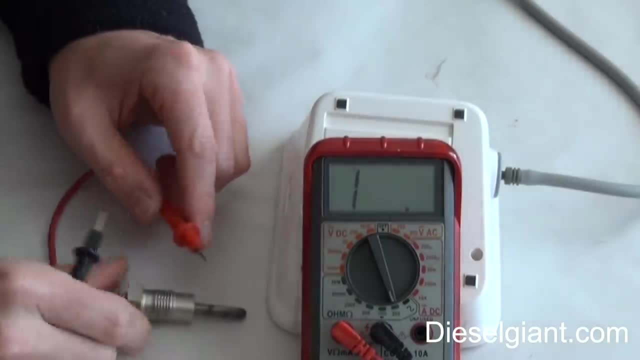 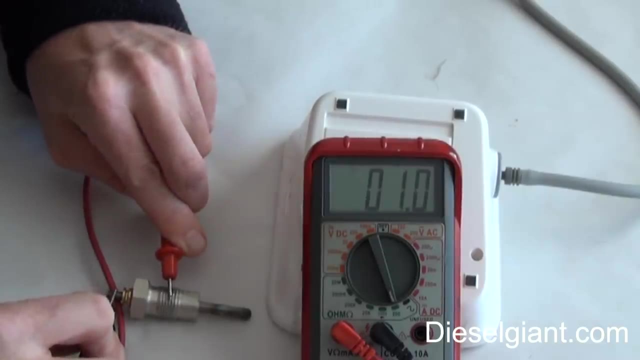 you to test your glow plugs. when you test your glow plugs, you're going to get a lot of resistance On your diesel engine. that's one way to do it. You could also test between here, where it's grounded, and here, and you get about- if I can hold it steady- about 0.9 ohms You. 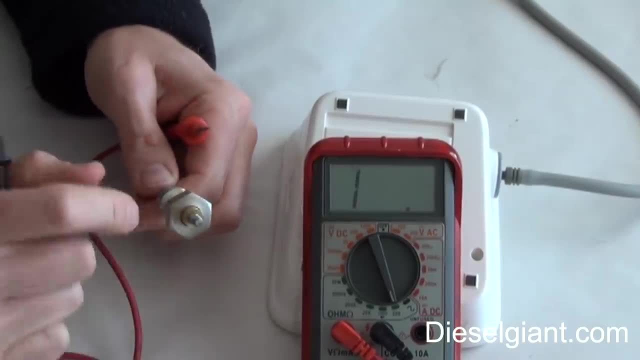 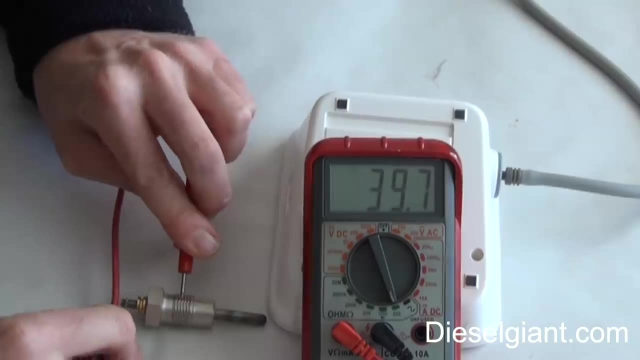 really shouldn't. if this is the power that's going in here and this is the ground, there should really not be any connection. There's a little bit, just because of the way I'm, I can't. it's hard to hold it still. 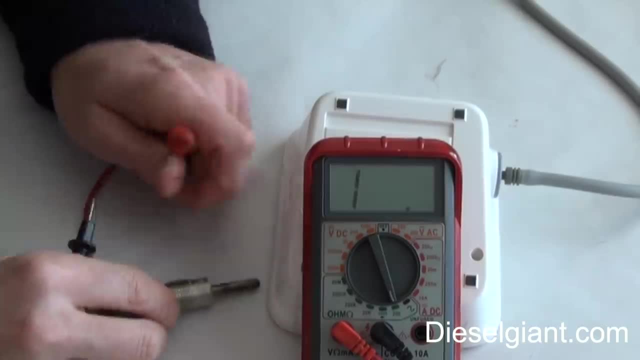 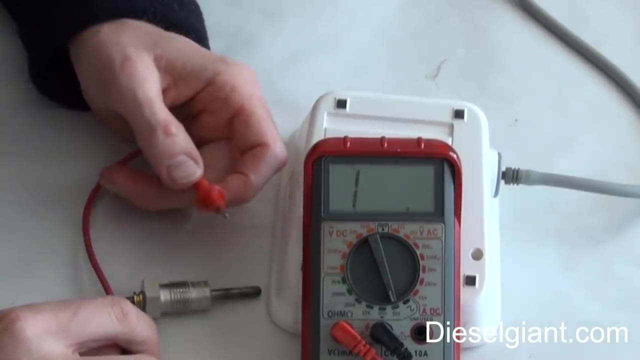 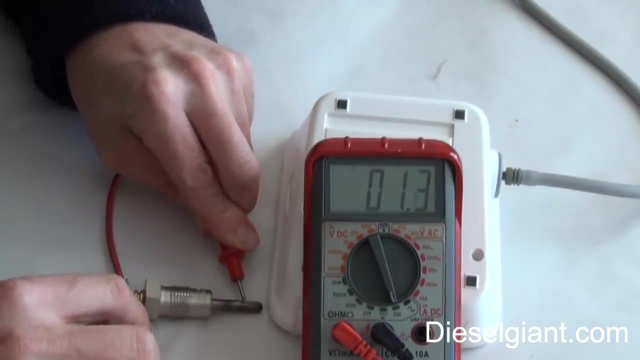 but if you wanted to test the element itself, well, let's just see. Now, let's say the element was broken inside. If it was broken inside, this is what I would get. You would see that it was open. okay, And again, the element itself is. it's about 1.5 to 1.2 ohms, which. 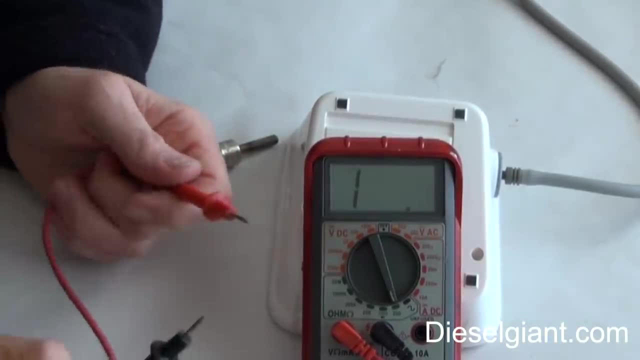 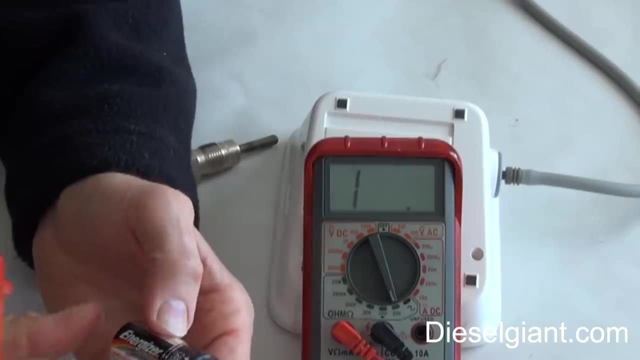 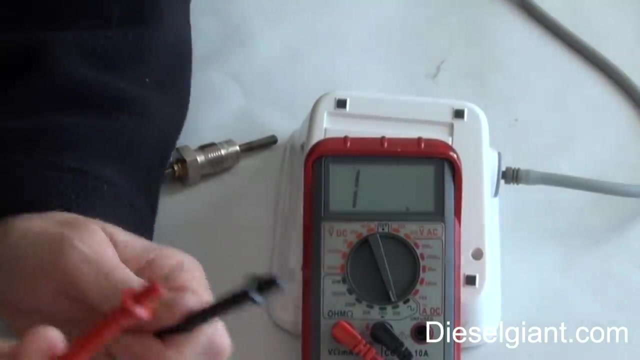 is fine, So you can go around and test things in your house. Just make sure. all right, I don't want to test the battery. This has got energy. As soon as I put the probes on either side here, it very well could blow this fuse out. Remember when it's in the ohms setting you're 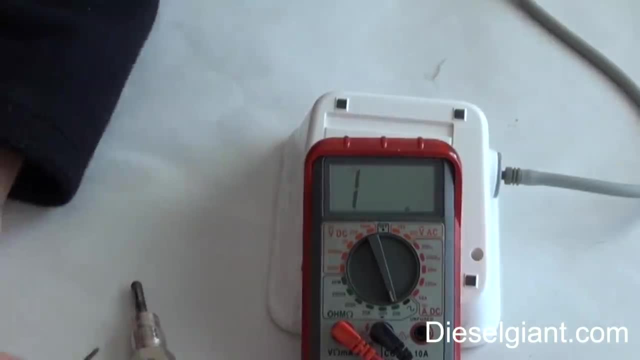 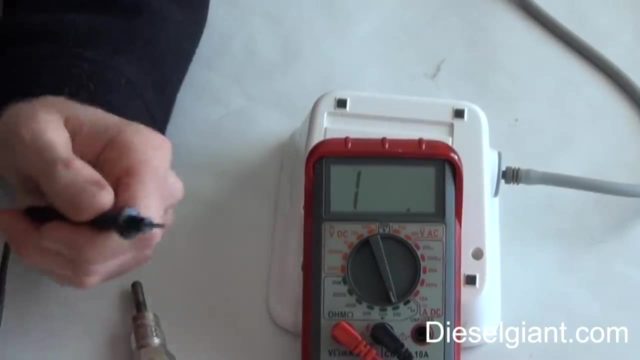 testing resistance, okay, So that's basically what you're going to use for automotive. You can test bulbs. you can test wires- Okay, You can test from one end of the wire to the other If it shows open like this. that means 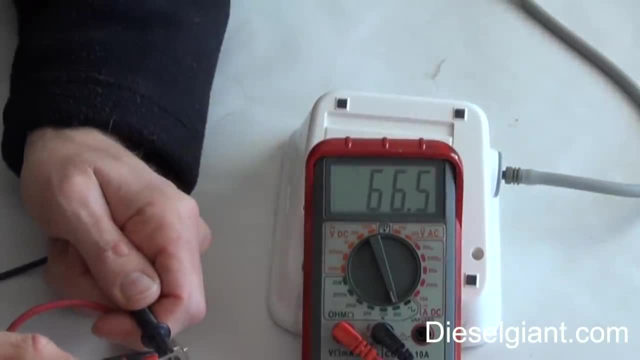 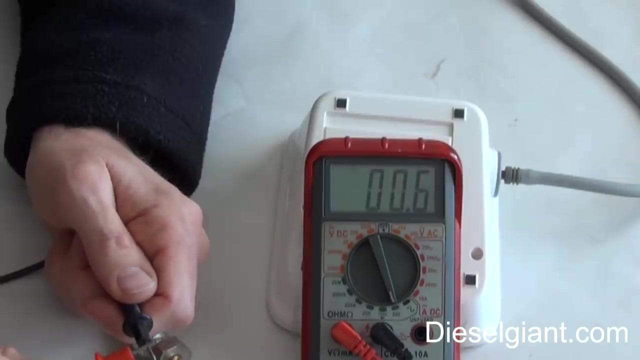 the wire has a break in it. If you see that the wire has, see there's no break. It's showing about point and it's bouncing around about 0.4,. okay, So we know that there is a path that goes from here into the meter and here The path is not broken If it's. 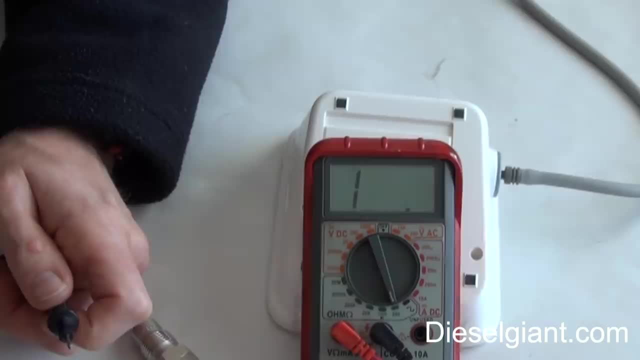 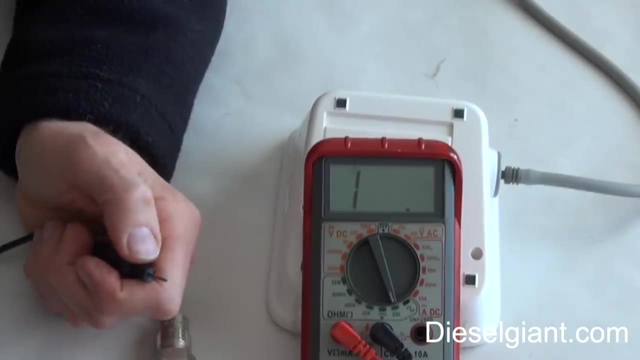 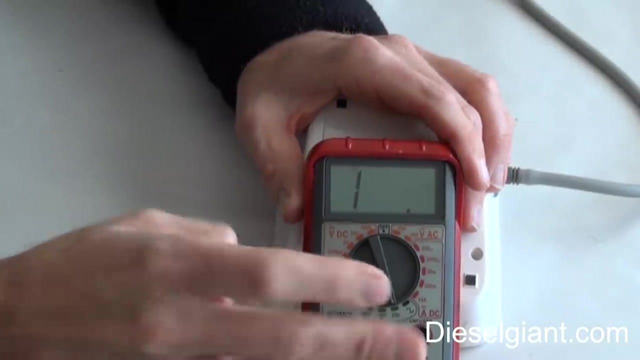 open. you're touching both ends. it's like that, then that means that the wire is damaged or something. So nothing is damaged between this end of the probe and whatever else you're testing on this end of the probe. So the bottom line of this video is not to be to show advanced testing techniques, It's. 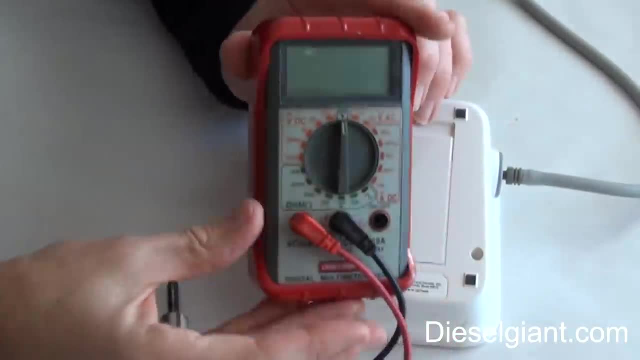 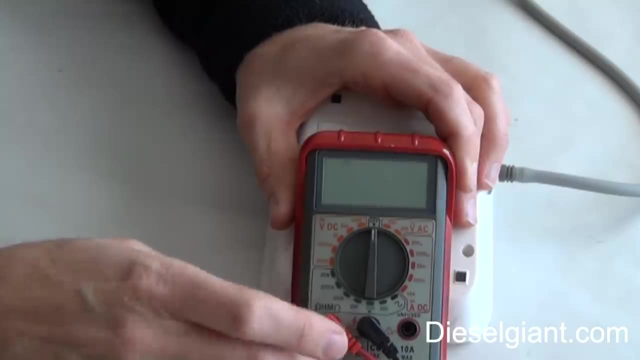 to get people that have never used a multimeter and they're scared of it to go out. get you a multimeter and this will allow you to do basic testing, like I've already shown you. So again, if you'd like to try to get this model- I haven't even checked it out, but 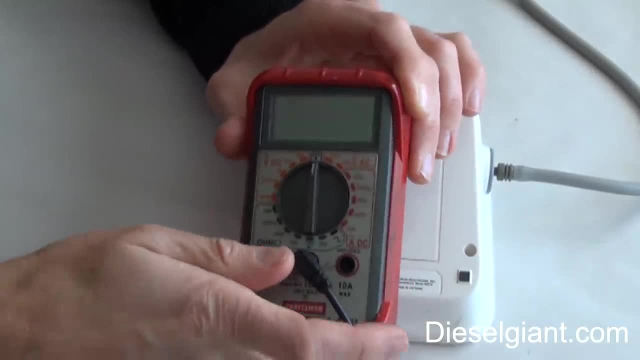 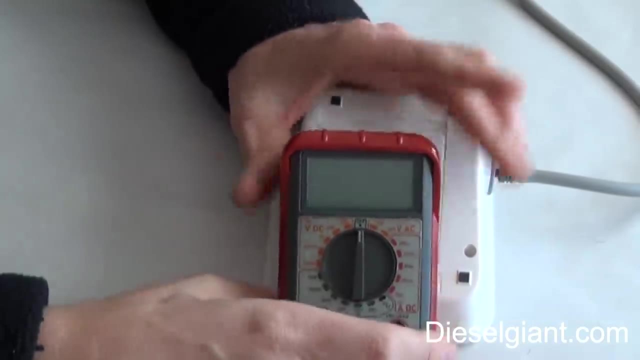 I've already checked on Sears to see if it's even available anymore. Sears does sell several different multimeters. Again, you can look and see what I've got on here. This is not the only multimeter I have, but this is the one that I. this is my workhorse, This is. 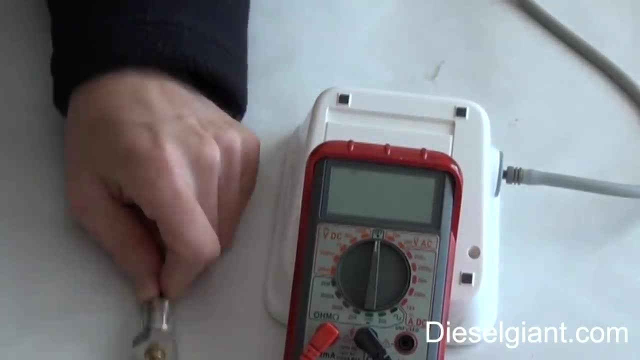 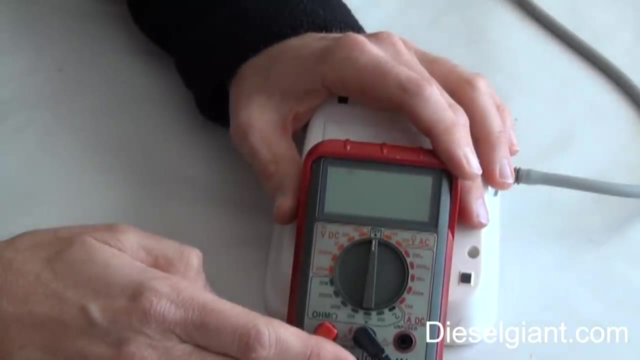 the one I use all the time and I do testing on glow plugs. I test batteries, alternators, just like I showed you to do on this video. So I want you guys to be able to get you a multimeter, utilize it and not be afraid of doing it. 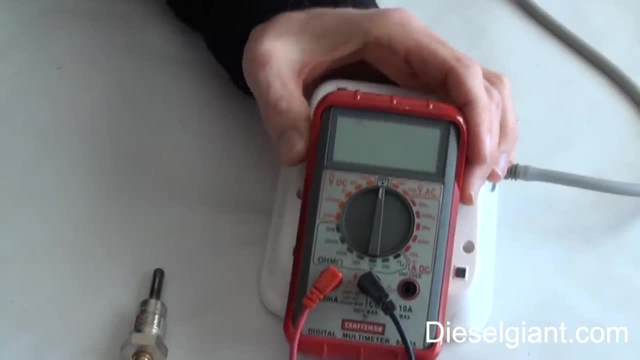 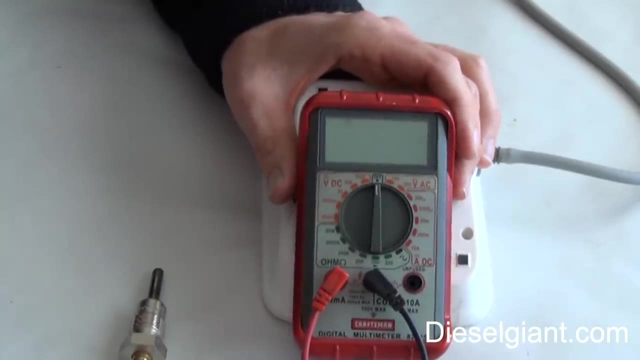 I hope this video has helped those that were intimidated by using a multimeter. If you have any questions, if you have any suggestions for upcoming videos that you would like for me to do, just leave a comment in the section below or send me an email. Contact me on. 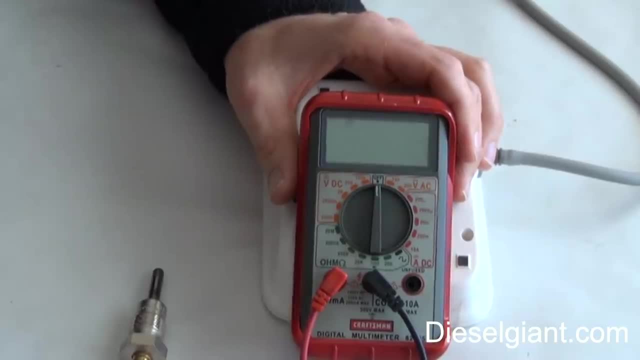 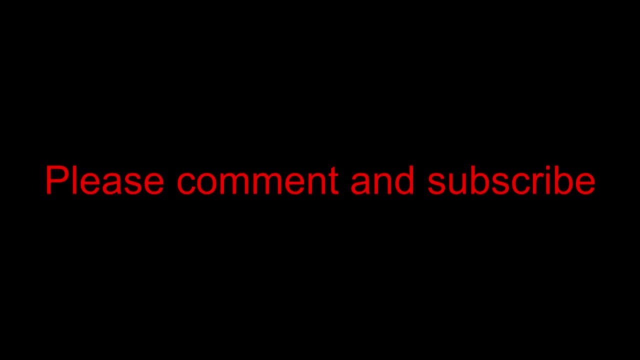 DieselGiantcom and I'll do my best to accommodate you. I hope everyone has a great and safe day. Bye.